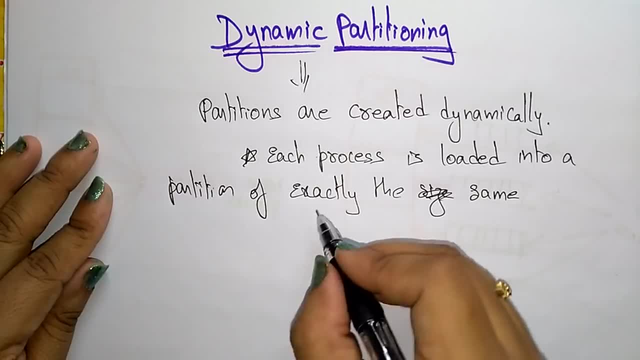 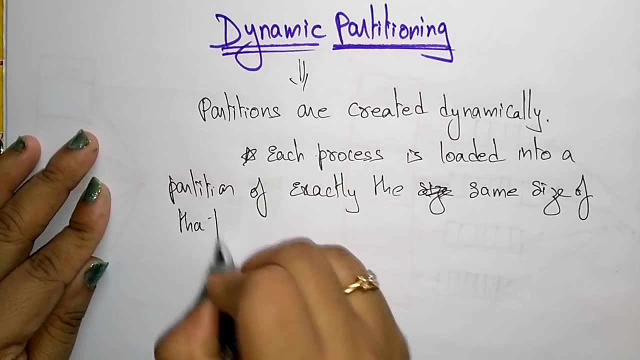 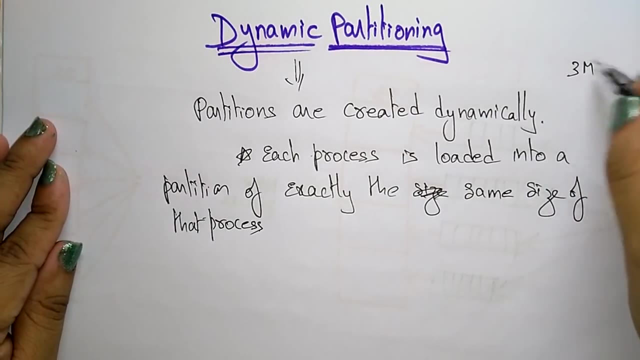 storing the process in main memory, the partition of the exactly the same size of that process you have to be chosen. suppose the process size is 3M, 3 megabytes, so it stores only 3M of memory. so you have to check in the main memory. 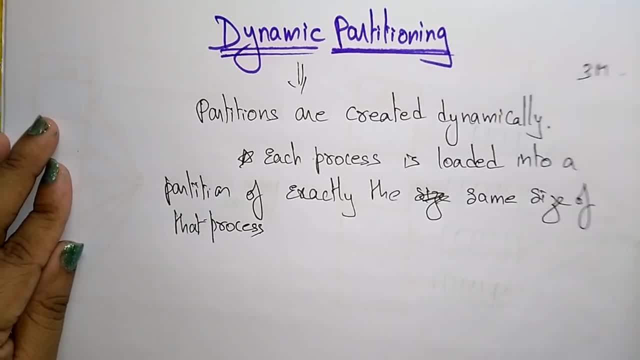 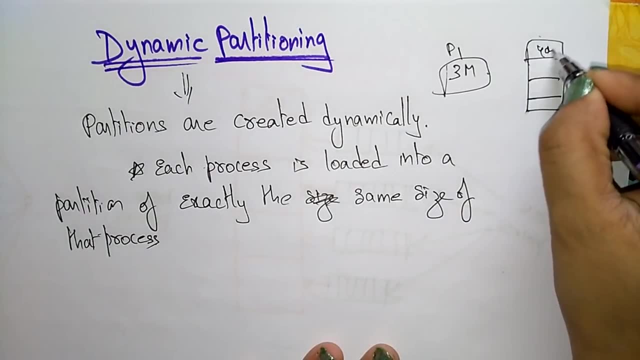 which is very close to the 3M. so in that memory location you have to store that, the process. this is a process P1, so suppose this is 4M and this is 6M and 8M, 12M, like that. so you have to store the process like this: 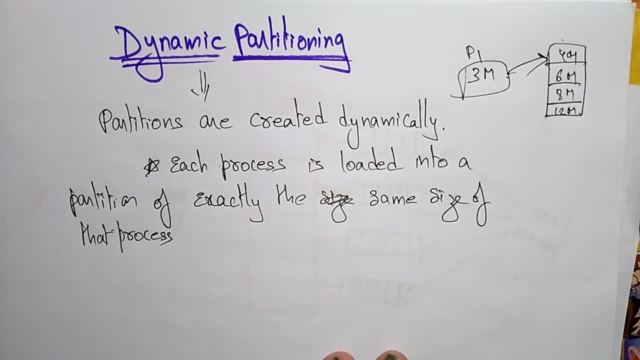 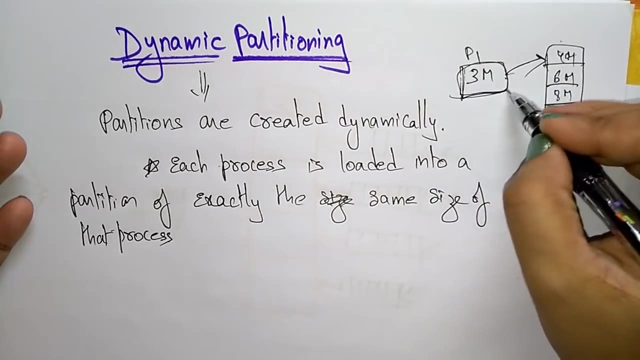 you have to store the process like this, have to store this 3m in this forum. so choose that type of slot, that type of partition, so that this- you call it as a dynamic partition- we are selecting so which is this process is fit in which partition, so that based on the selection. so that's why we call it as a dynamic partition. 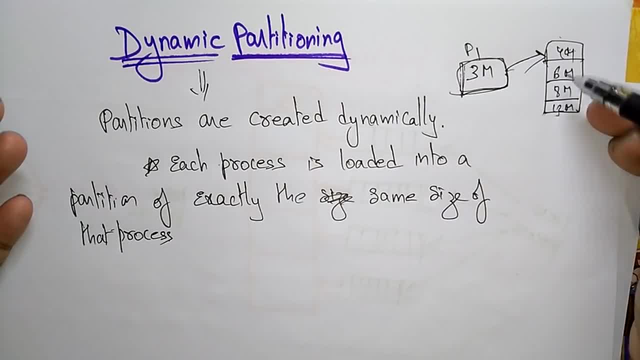 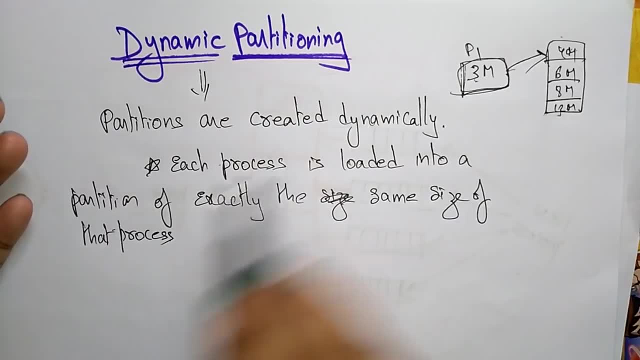 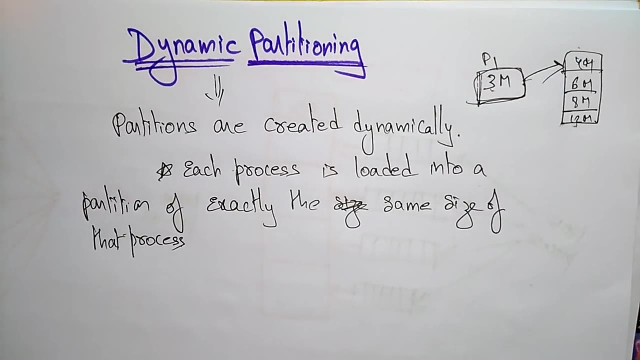 not. we are frequent serial, we are storing random. here we are storing the process randomly, so each process is loaded into a partition of exactly the same size. it should be exactly the same size, or each it it should be nearer to that same size of that process. so this technique, you 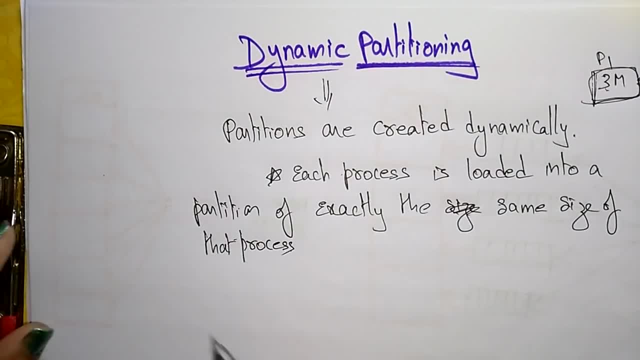 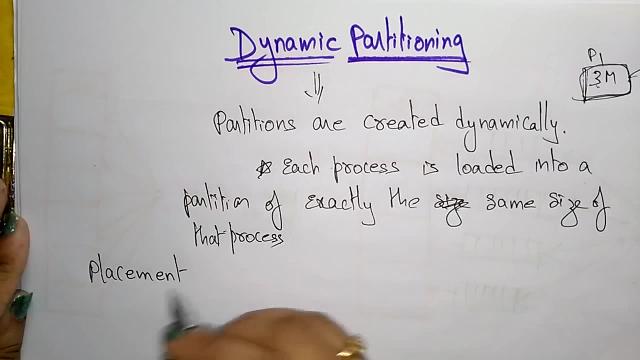 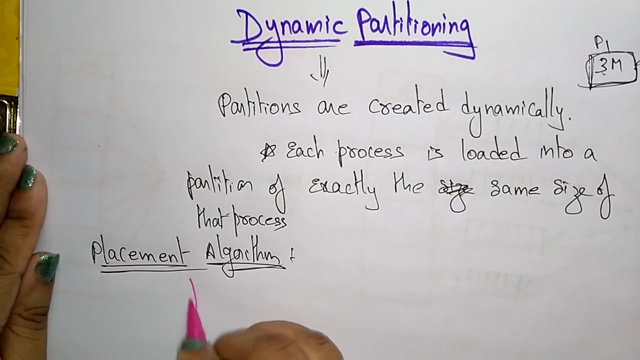 call it as a dynamic partition. so here we will use some placement algorithms. so how we have while you are placing the partition or while you are placing the process in a partition, so you have to know about the placement algorithm. so while placing the process in main memory, you have to think about the first fit. 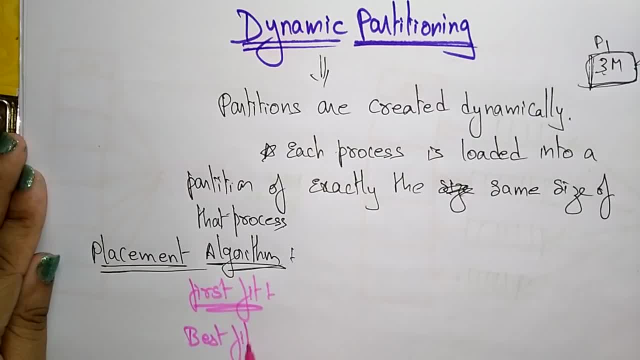 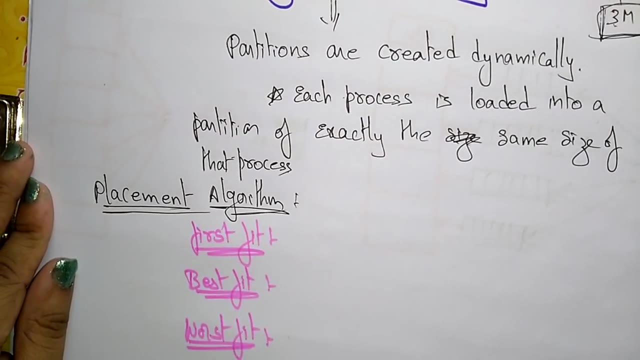 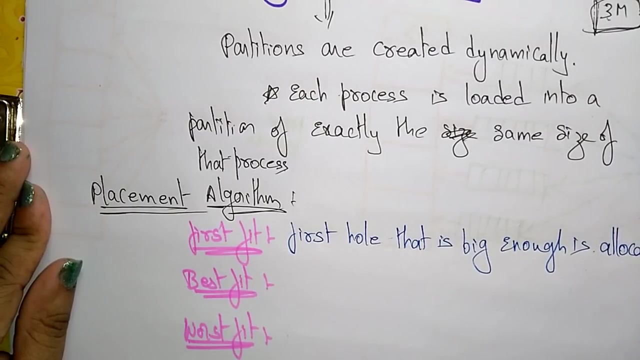 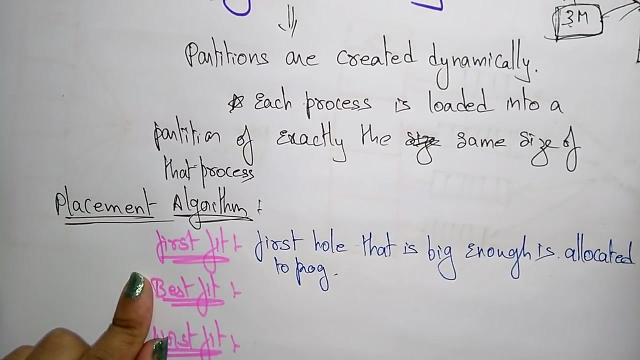 next best fit, next worst fit. so the placement algorithm of dynamic partition may be a fast fit, best fit or worst fit. so first fit means first hole that is big enough. the first hole that is big enough is allocated to program. so here they are saying that the first fit means we have to first. the first hole means the first. 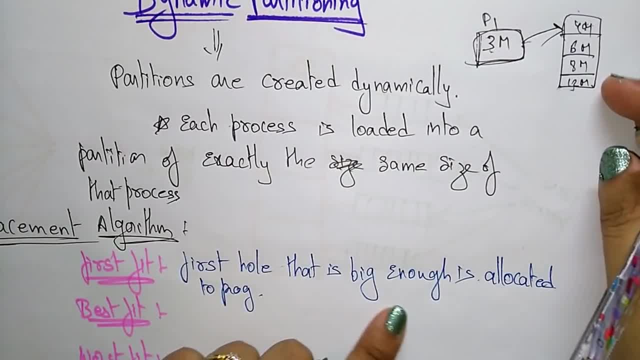 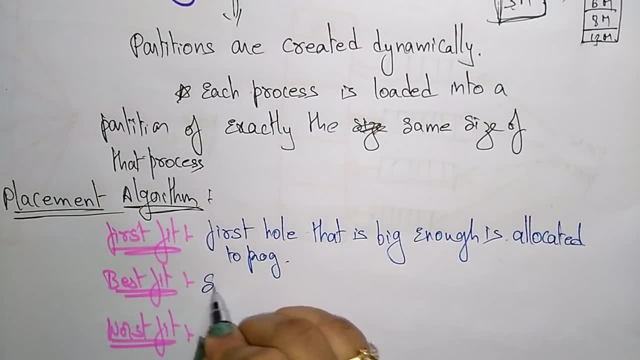 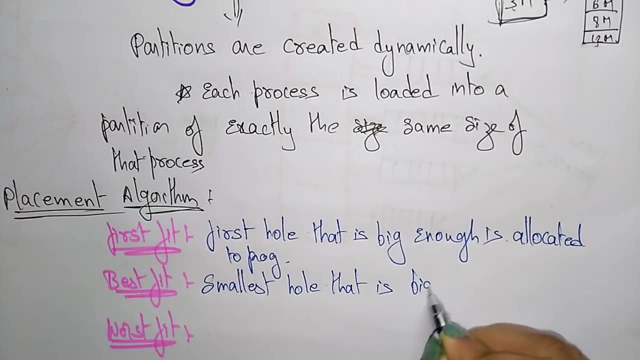 partition, the partition that that is big enough is allocated to program. that you call it as a first fit. now coming to the best fit. best fit means smallest hole that is big enough is allocated to program. so this is best fit means you have to select the smallest hole. that is. 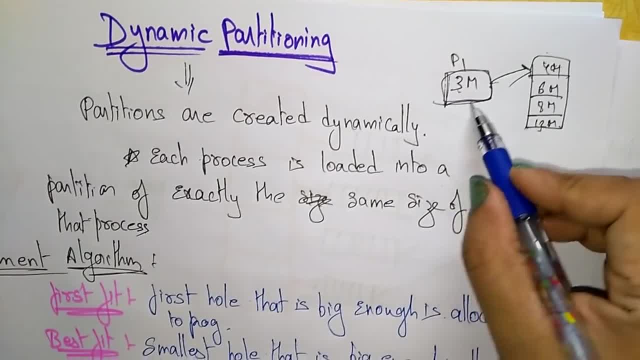 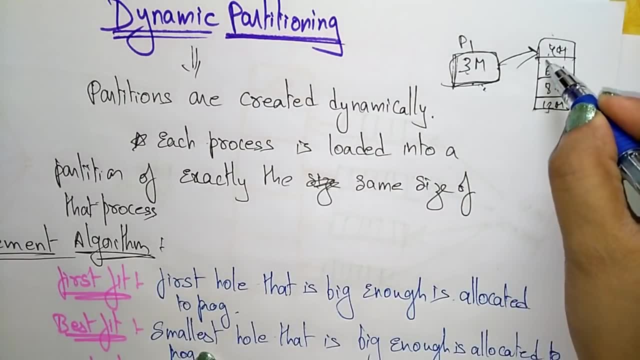 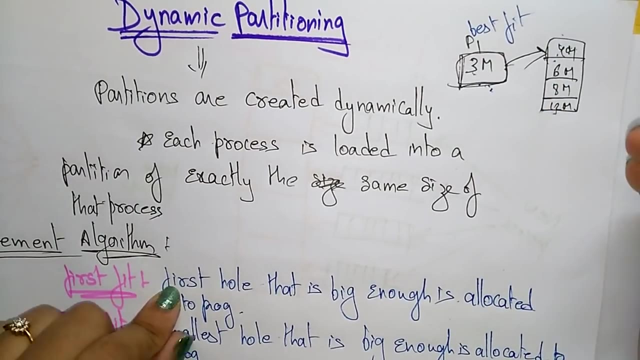 big enough is allocated to program this. i here. whatever i explained here in this example, this is the best fit because i selected the smallest hole which fit for this process. then you can say: this is best fit. means here: uh, not uh. more space is wasted in the first means. 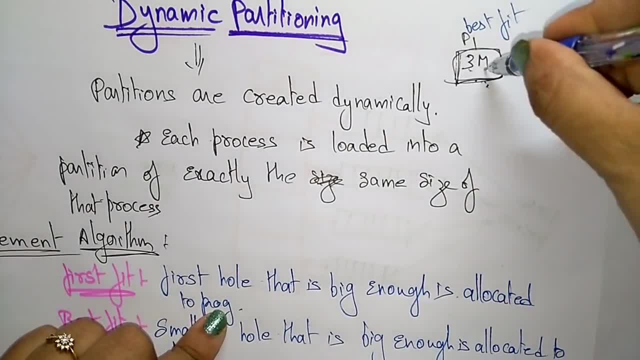 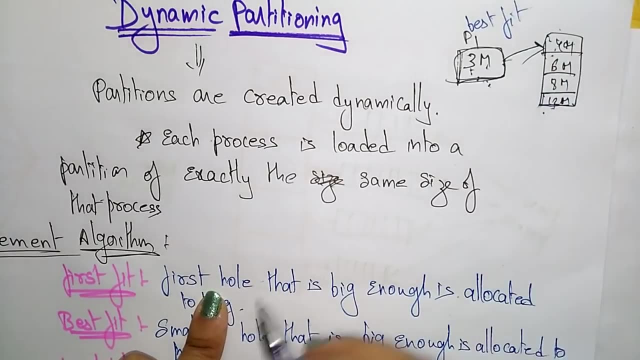 the first hole that is big enough is allocated means you have to store the 3m in 12m. suppose. if you store store this process, uh, in 12m partition, then you call it as a first fit, not not first fit, first hole. oh sorry, sorry, the first hole means the first hole that is big enough. so which is the first? 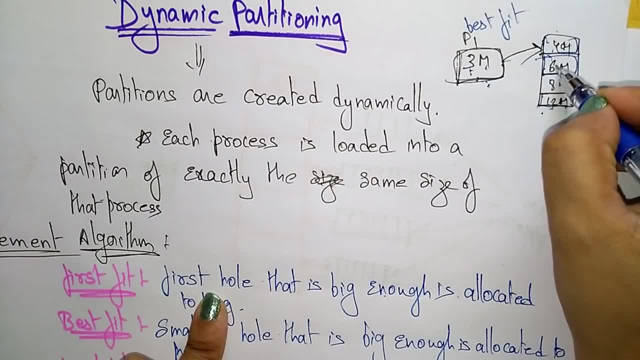 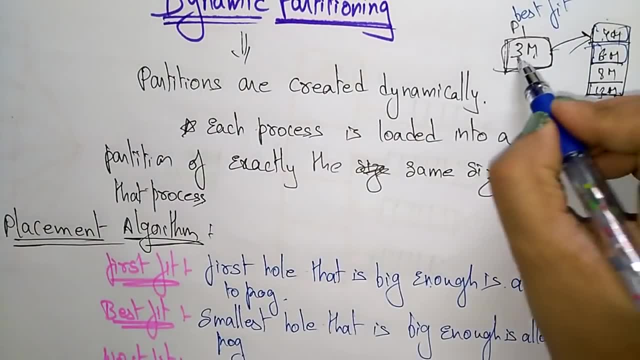 hole that is big enough, that is a 6m. so he, if you store here in 6m that you call it as a first fit, now coming to the worst fit. so worst fit means whatever i said, the 3m is, process in 12m, the large. 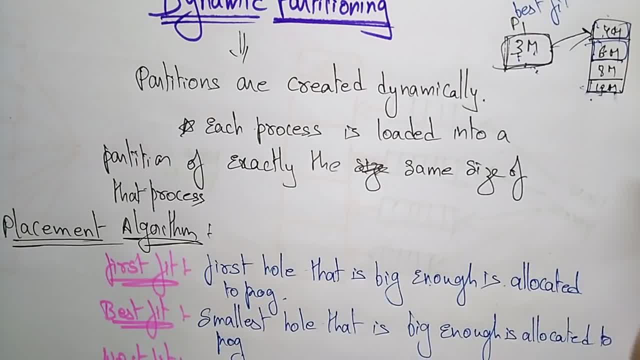 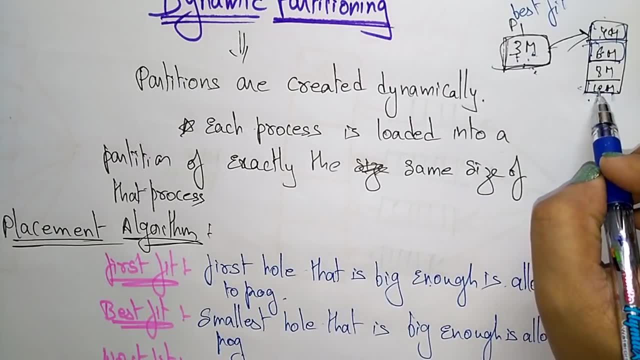 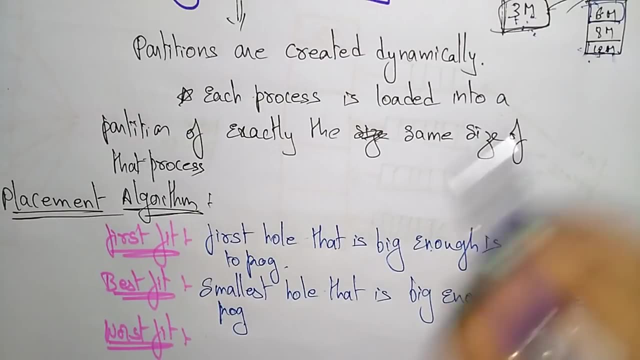 enough large hole that is present in the memory, main memory, large partition. if you store that single process which is the size less than that of partition that you call it as a worst fit, because there a lot of memory will be wasted. so that's why we call it as a worst fit. worst fit means largest. 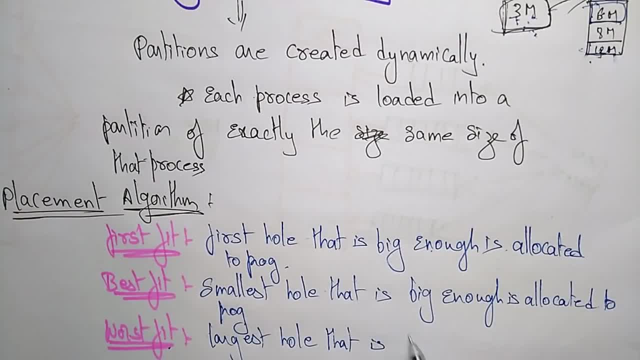 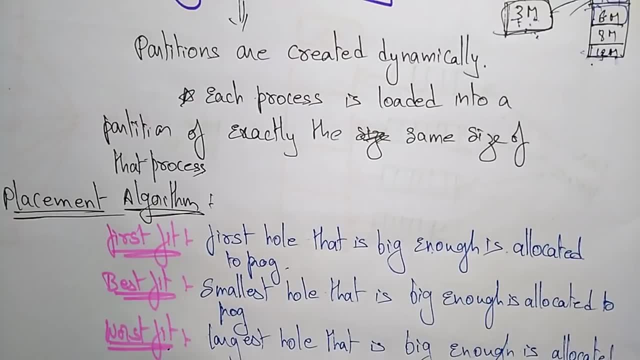 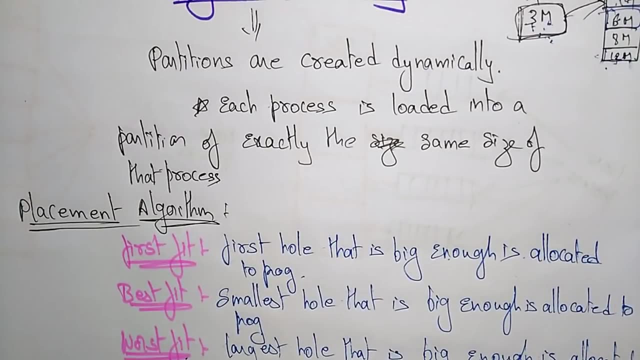 hole that is big enough is allocated to program. so this is, this is a placement algorithms for the dynamic partition. so why, while you're placing the process in main memory by using dynamic partitions, you have to think about whether you are using the first fit, best fit or worst fit? 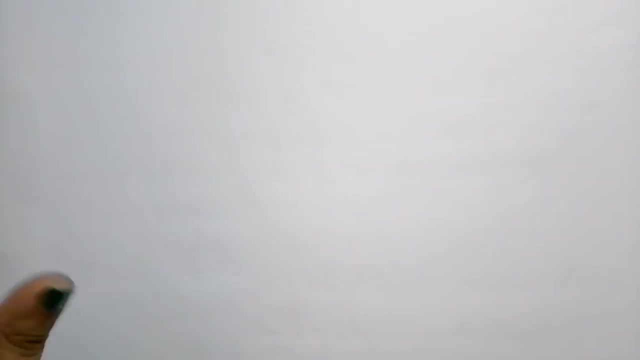 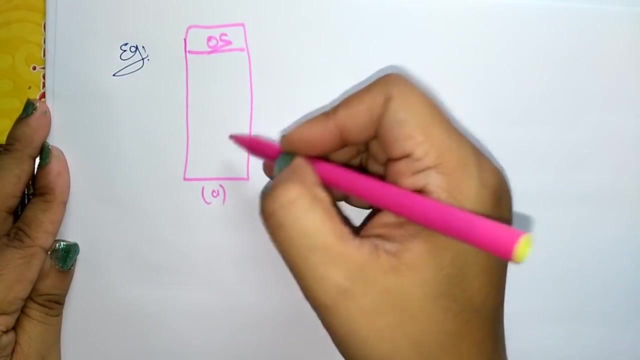 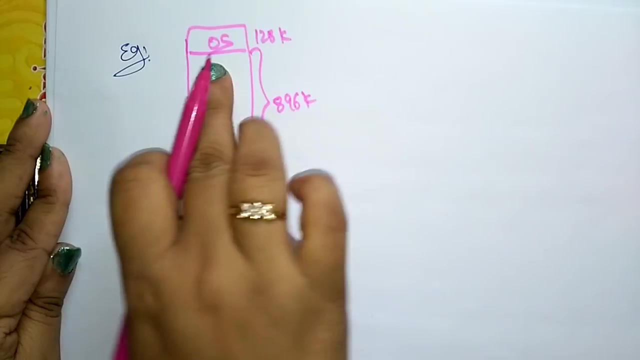 so let me explain that by taking an example, so how the process will be allocating dynamically. here is the example. suppose, if we take first one here, the operating system and the remaining complete here, uh, the complete, uh main memory is occupied by one process, 96k, suppose the size 128k is allocated to operating system and the remaining complete process is: uh stored in the rest to instrumentation. if we are applying dynamicct we can see that here main memory will be saved to operating system and the remaining complete process will be stored in the rest to Luther memory which will take care of his life. size andystem here causes memory removal. 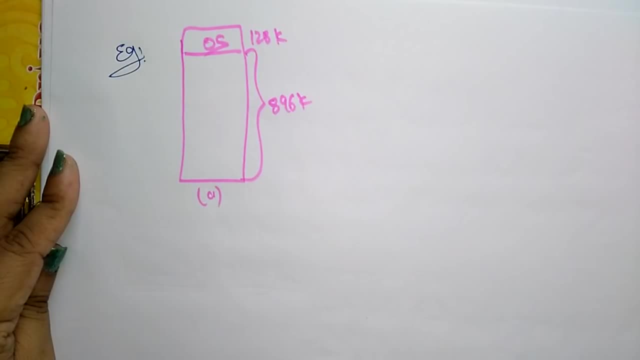 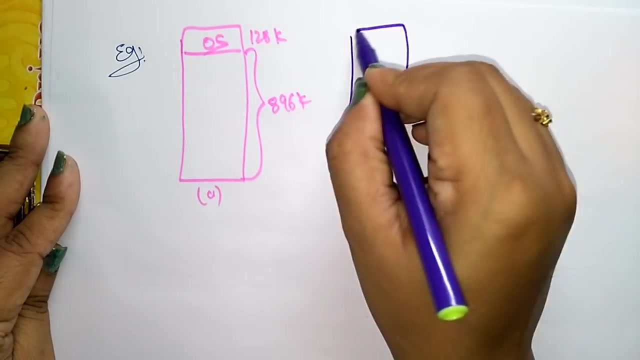 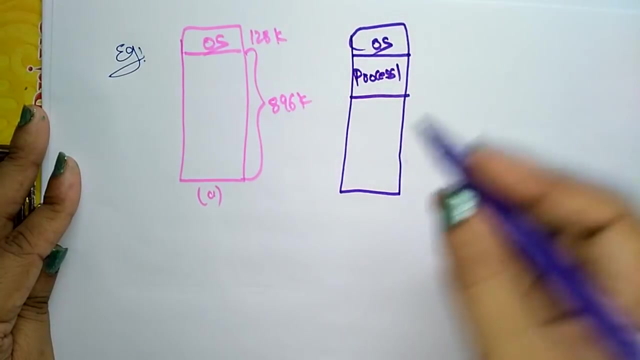 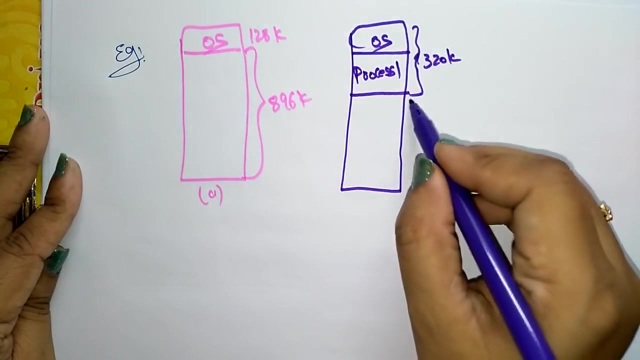 Stored in the rest of the memory. So this can be. this is one of the dynamic programming, So this you also call as a dynamic programming. Or else you can store first the operating system, the process one is stored in. so this is completely 320k. you are taking only 320k and the remaining will be empty. 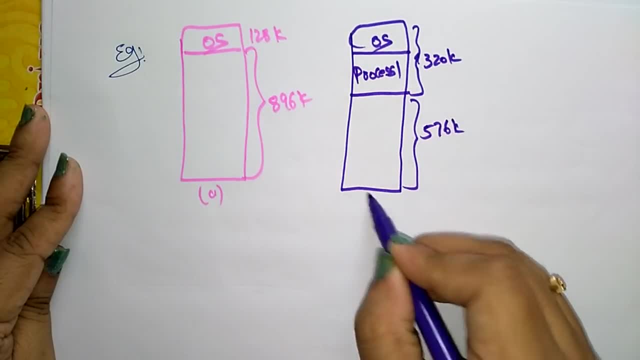 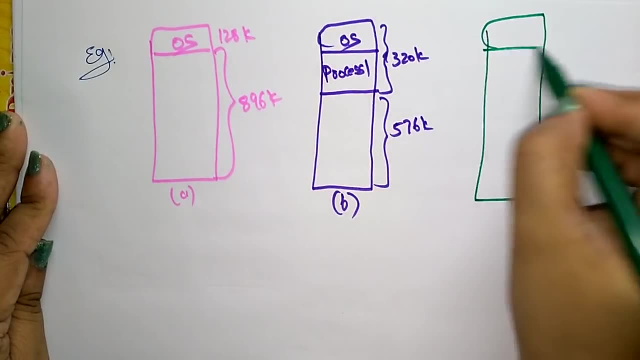 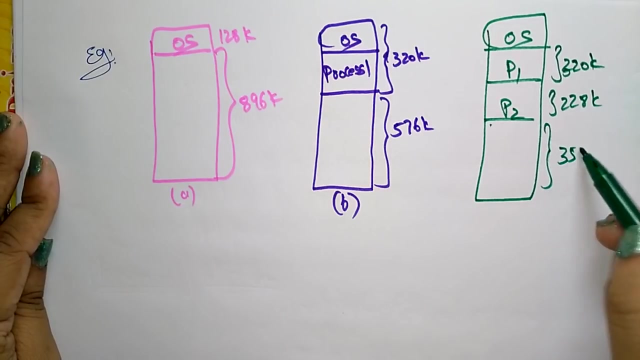 Okay, So this is one way of storing the process in memory, or else you can take like this, the operating system, the P1 process, P2 process. So here the P1, suppose it is occupying 320k, and this is occupying, suppose, 228k, and the remaining, suppose 352k, is empty. 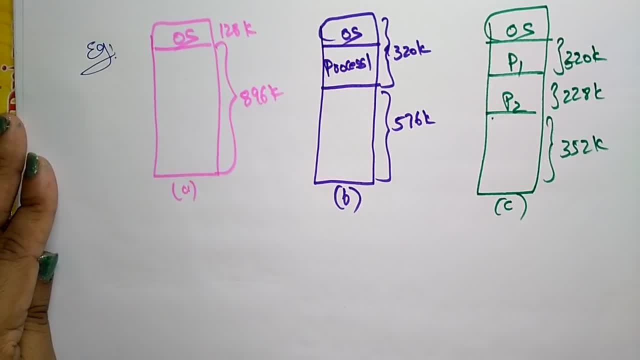